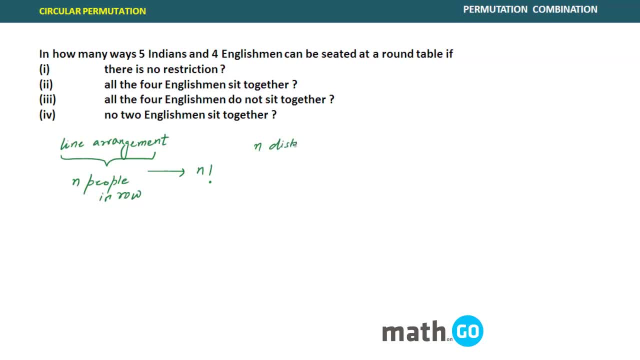 right. So for n distinct objects: when n distinct objects are to be arranged in a circle, right they are to be arranged in a circle, the answer becomes n minus one factorial right. So this is how you have to remember. So for here it was n factorial, here it will become n minus one factorial. So let me show you, with the help of an example, that why we are doing n minus one factorial right. 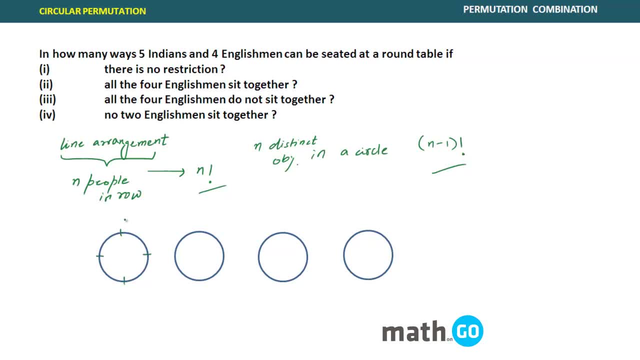 So let's say there is a circle and I am trying to arrange four people in a circle, right, Let's say I see to them like this: a, b, c and d. then I rotate them in a clockwise fashion So they should become sorry. this will be a here, right, this will become b and this will be c. rotate them again. So this position will be held by just do this activity. So these are the four particular positions that I can draw. 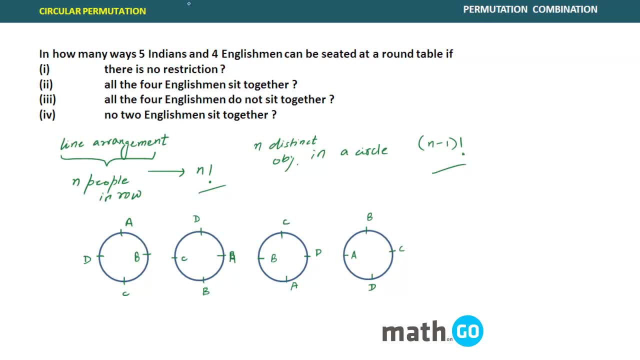 For the circle. Now, in case of line arrangement, since four people are there, so in case of line arrangement there would have been four. factorial answer, that is, you can say 24 arrangement would have been there in case of row. Now what will happen in case of a circle? So, for a circle to become a line, what we can do is we supposedly cut it from here every time. right, you cut it from here. So if you cut it from here, this thread would look something like a, b, c, d, which is one arrangement in row. this would be. 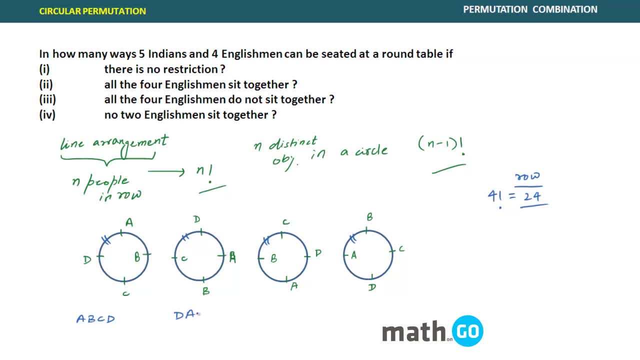 start from here to go to the end of the thread, This will become d, a, b, c, completely different arrangement from this. Now let's talk about this. this will become c, d, a, b, right, and this would want to become yes, b, c, d. So these are the four different line arrangements which actually become one. they become one in case of got it, in case of circular permutation, In case of 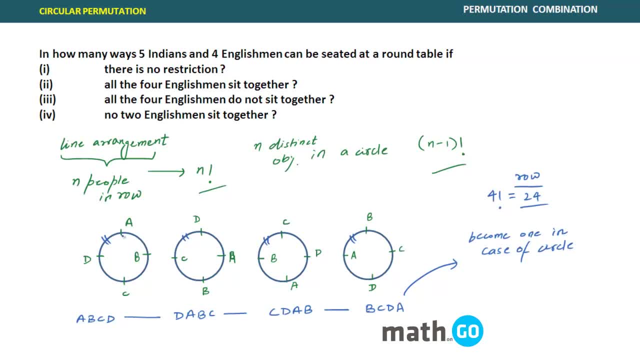 circular permutation. they are all one. Why? Because, anyway, you see the left in circle, what you see left and right, who is sitting to your left, who is sitting to your left? So always a has left and right as d and b, c to it in all the four diagrams. So that means all these four cases were reduced to one, or in fact you can say your answer to this problem was reduced by four. So what is four factorial? by four, that is nothing but three factorial. If I analogically apply this, if there 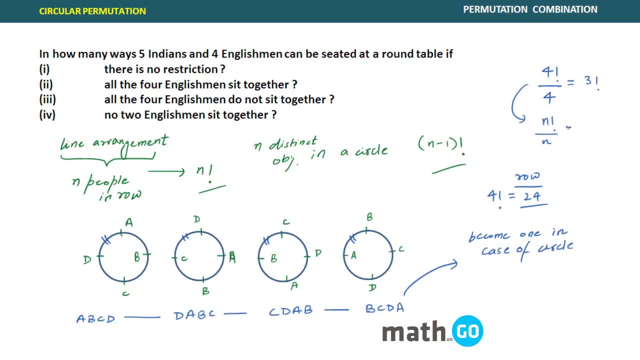 was a n people in a row, your answer will get reduced by n. this becomes n minus one factorial. So this is how you actually derive the formula for circle. Let's apply this now in a particular problem. The problem says in how many ways five Indians and four Englishmen can be seated in a roundtable conference. And these are the four questions. So if there is no restriction, so how many people are there? There are nine people, or nine people to be arranged in a circle. 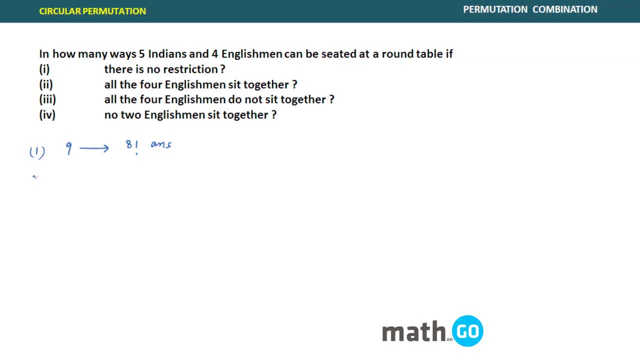 The answer would become eight factorial. So this is the answer for the first part. very simple stuff. Let's talk about the second part. All four Englishman said together, right, So you want all the Englishmen to sit together. so we have done the case of questions where some people sit together. So what we will do will from a group out of them, microwave. remember in the previous lecture I did so. that means rather than saying for Englishman, I would say this is one Englishman, right, one people. and there are 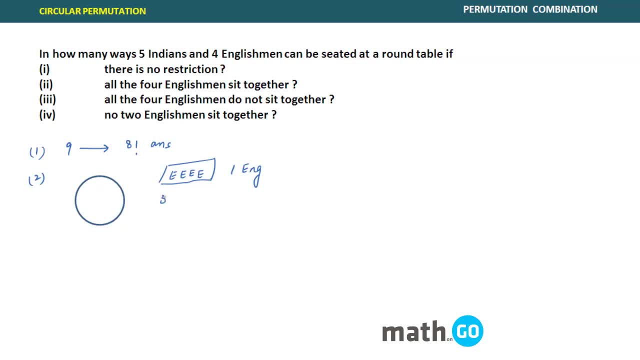 five Indians. so that means you in total there are. there were five Indians in macro. you what I'm seeing? one Indian plus this one Englishman. they are total of six people to be arranged. six people to be arranged in circle right. so how we can do that? yes, we can do that very easily. in how many ways? 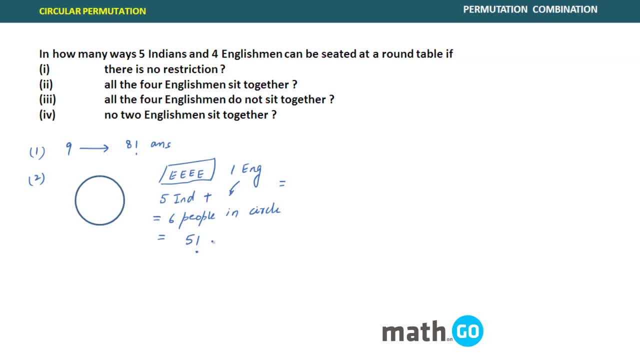 tell me five factorial ways, but this is not the answer. this was the answer for the macro view. but what about this component? we have Englishman which are seated common. the answer to this particular problem, then, will become five factorial into four factorial, because the four Englishman can be seated in. 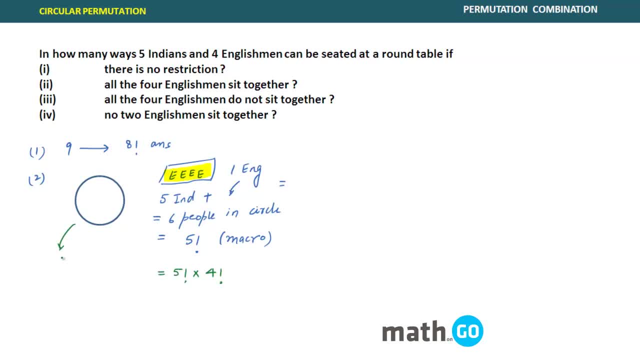 four factorial ways. mind you, some student here actually answer this particular answer, five factorial into three factorial. what they do? they try to arrange four Englishman again in a circle. never do this activity. so when you have answered this five factorial, that means you have drawn them on a certain, drawn a circle already. 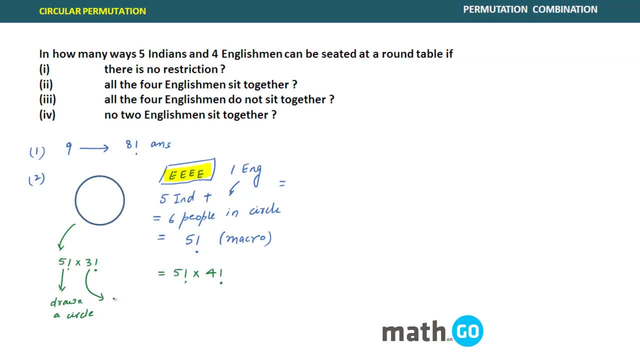 right. so the next answer of agreement will never be in a circle, will never be a circle. you just remember it. like this circle will be drawn only once. you cannot draw a circle twice. so for all other arrangements you will follow. now line arrangement if a circle has been drawn. 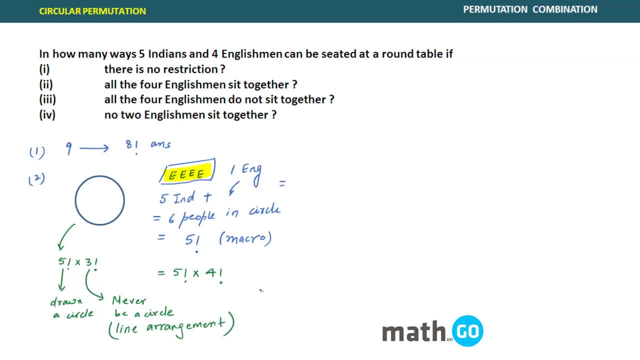 you will now only follow line arrangement. you will not follow what I call as a circular arrangement. so five factorial was has already taken into account your circular arrangement. the next would be four factorial. so this is the answer. reject this answer. this is not the correct answer, remember. 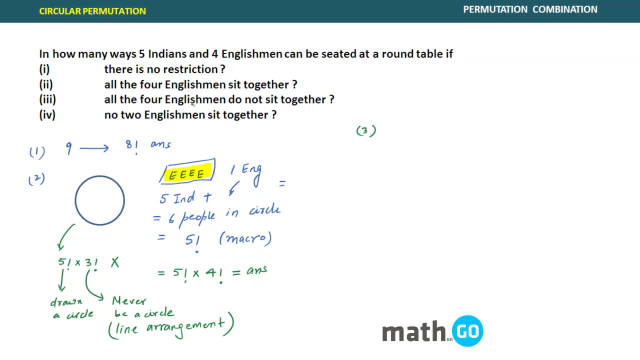 let's take the third component. says: all four Englishman do not sit together. so now something of very different. let's see how would you apply it. so very interesting problem. it says that all four Englishman do not sit together. right, so let us talk about that group. 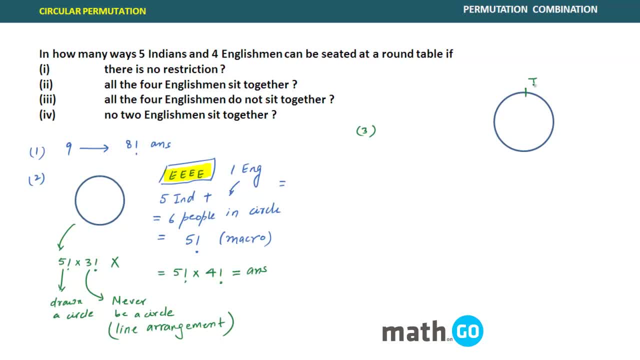 which on which there is no condition. so Indians do not have any condition. to first of all, let the Indian be seated in the circle right. there are how many Indians? there are five Indians right. so five Indians have been seated in the circle and for a circular arrangement, five people can be seated, as into four factorial ways got. 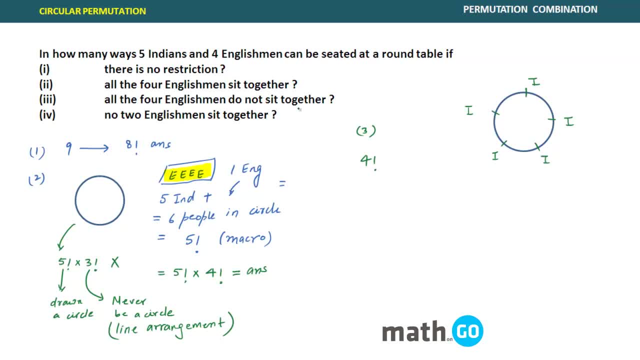 it clear now: you want no four Englishmen to sit together. that means between every Englishman there should be an Indian accepted. so remember the dash problem that I did in yesterday lecture: how many dishes can be drawn there? five positions. and if any of these five positions are taken by the Englishman, they were always fine. 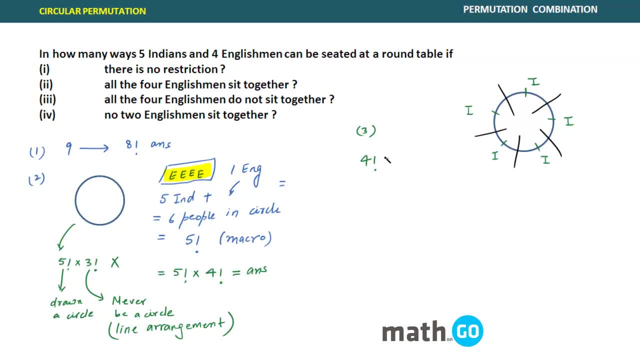 and into the left and right, remember. so out of these I can say there are five positions and there are for Englishman's or five you have to select. for first of all, let's see if I say English, one here, Englishman to Englishman, three here and Englishman. 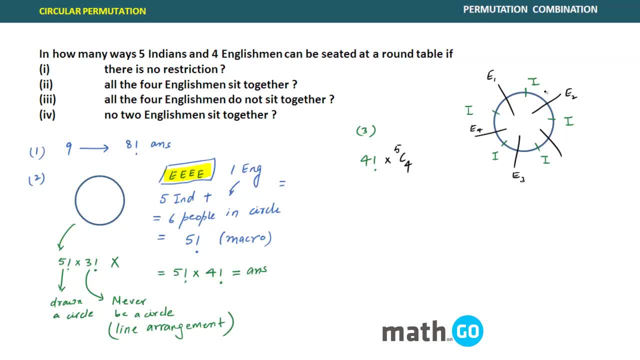 for here. see any two Englishman. there is always an Indian between. do not worry about serve. these two Indians are sitting together. it is not given in the question. we wanted two Englishmen not to sit together. where is it it could be possible that Indians will sit together? 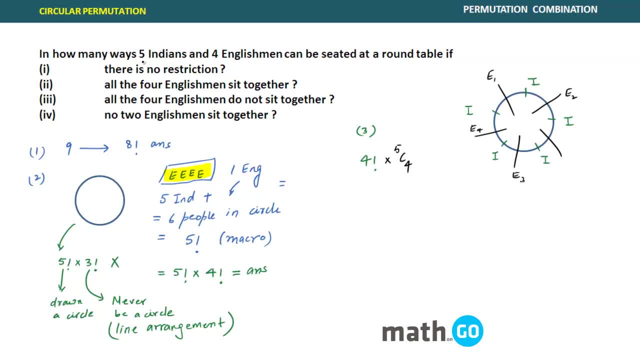 and I told you yesterday also, if the numbers are not balanced, that is, one is greater than the other, obviously one group will have to sit together. if this is the answer, if this is the case, and then they could also arrange them. so in how many ways the Englishman will arrange? 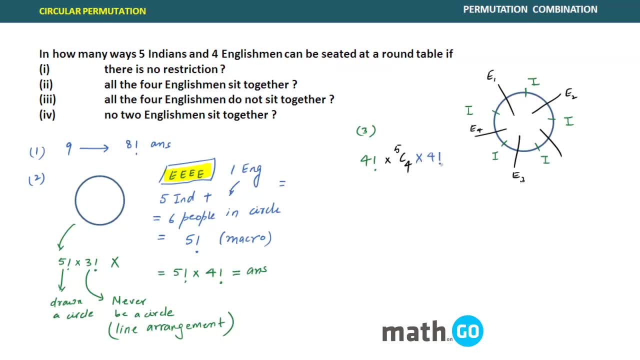 three factorial or four factorial. remember they will again arrange them in four factorial ways, not three factorial. we have already drawn the circle here. keep this in mind. so this is the answer we are looking for in this particular problem. let's take the fourth one. the fourth one says no two Englishman sit together. 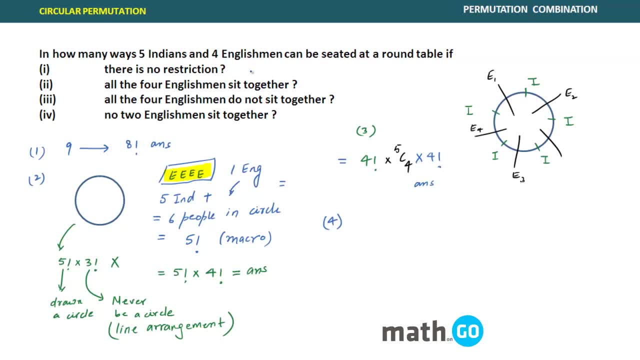 okay, okay, my mistake. first of all, the answer that we have just solved is actually: this was not the third one, it is the fourth one, when we say that no two Englishman sit together. now let us solve the third one, where they say that all four Englishmen do not sit together. this is what we have already solved, this. 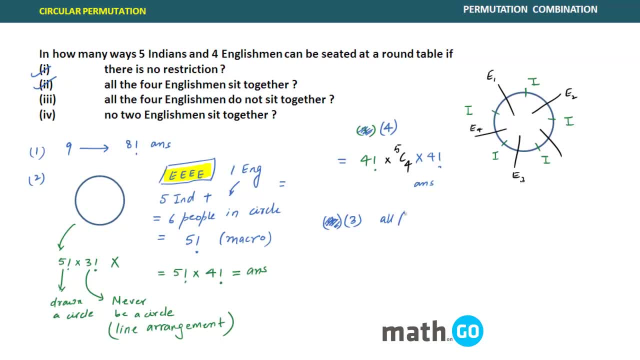 is the component of first and second. so all four do not sit together. it is what we have already solved. do not sit together, right? so what we can say when all four do not sit together is total cases, right, minus those cases when they sit together, and this is what we have actually solved in part 1 and part 2. so 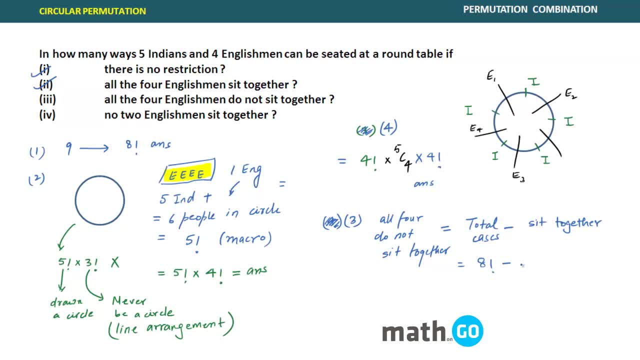 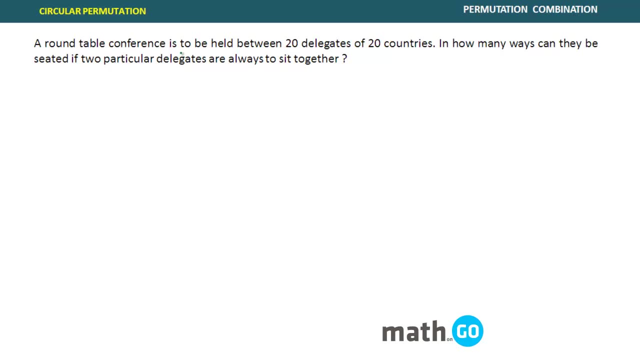 the answer is nothing but 8 factorial minus this particular answer, that is, 5 factorial into 4 factorial. so this is the answer to this particular problem, right? let's take another problem on circle permutation to understand it better. it says: a roundtable conference is to be held between 20 galley delegates. 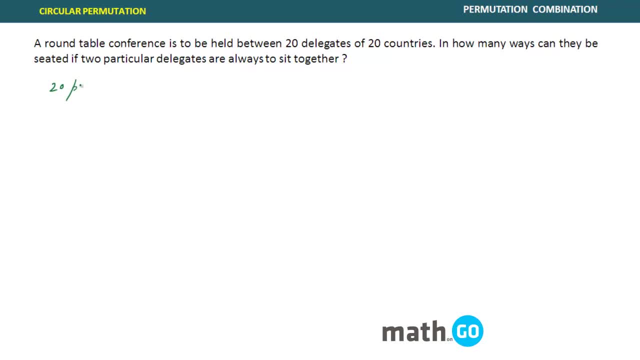 of 20 countries, so there are 20 people for me. right, delegates of people are one in the same thing, so there are 20 people for me in the roundtable, so they are seated in the round table. in how many ways they can be stated, if two?